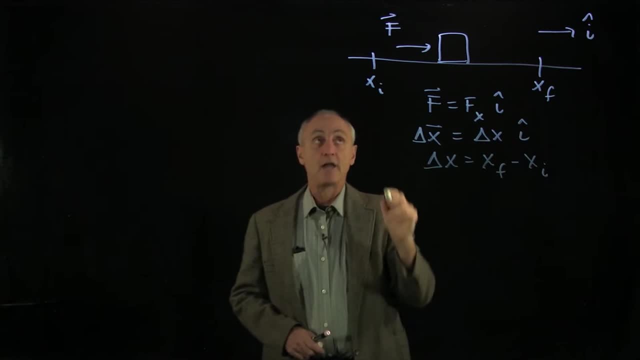 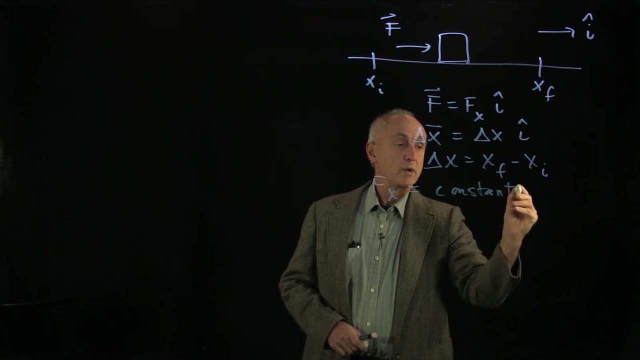 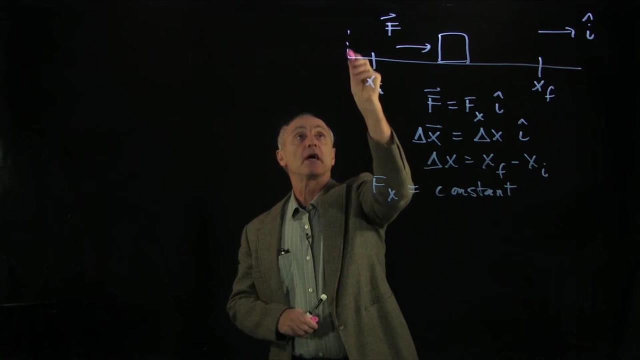 equal to x final minus x initial, And for our constant force, for the case where fx is a constant, We would like to define the work done by this force in displacing the object from our initial position- and we'll mark it like that- to the final position here. 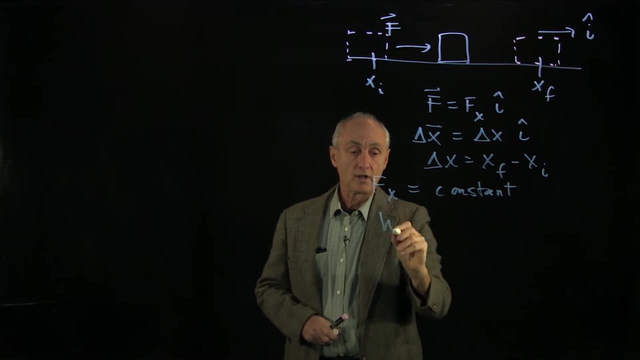 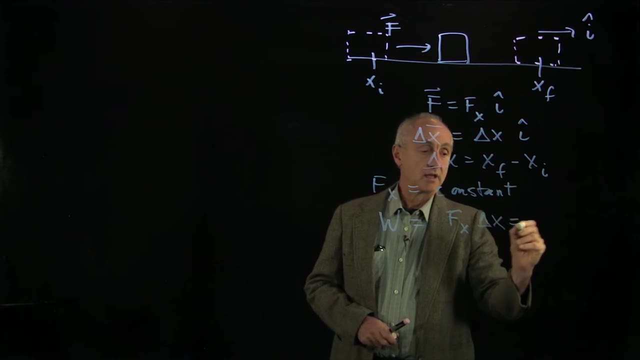 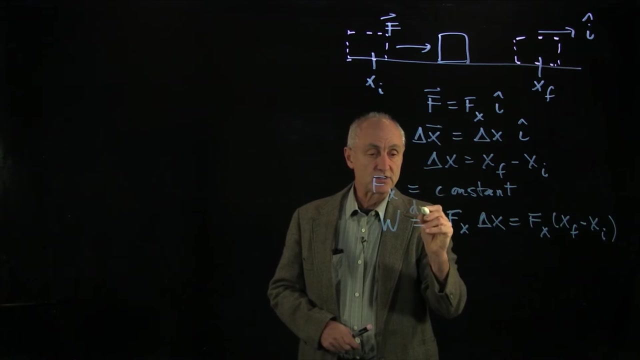 is given by the product. So we'll call work is the product of the force. fx times the displacement And so that's equal to fx times x final minus OK, That's x initial And this is our definition for work for the special case. 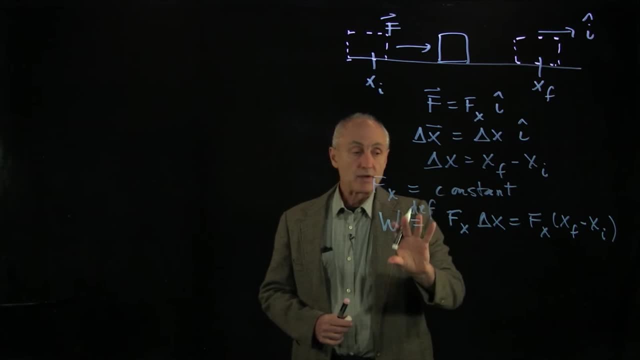 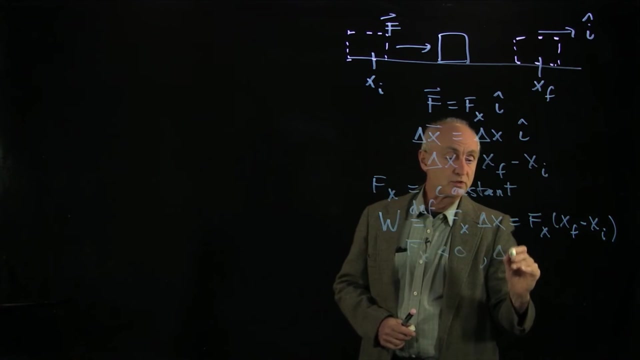 where the force is constant. Now, if we look at this, our force may. in our diagram we drew it in the positive x direction. But if our force fx were less than 0 and our displacement was in the positive direction, positive, 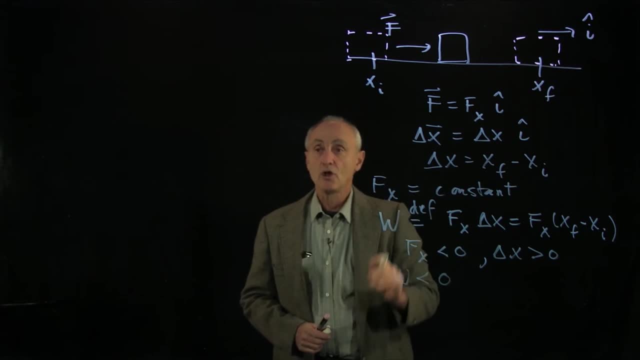 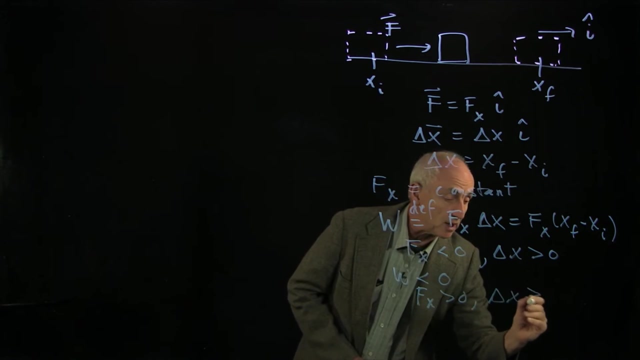 then you can see that the work is negative. If the force is opposing the displacement- and that's what would happen if fx was pointing in the negative direction- the work would be negative. If fx is positive and the displacement is positive, then the work is positive. 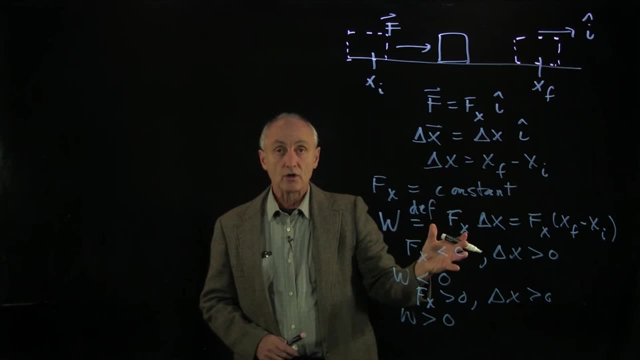 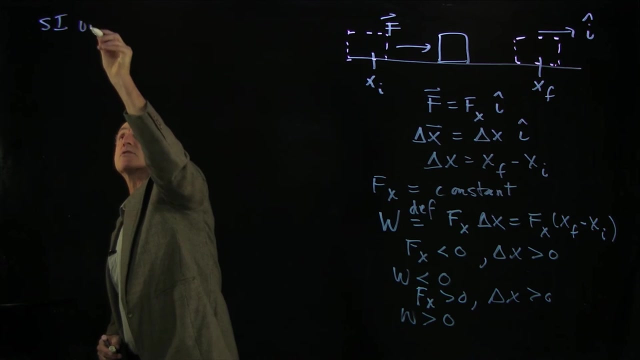 So we see work is a scalar that has assigned quantity, positive or negative. Now, whenever we introduce a new quantity, we always have to be a little bit careful about the units, since work is the product. So force and distance. then our SI units for work: 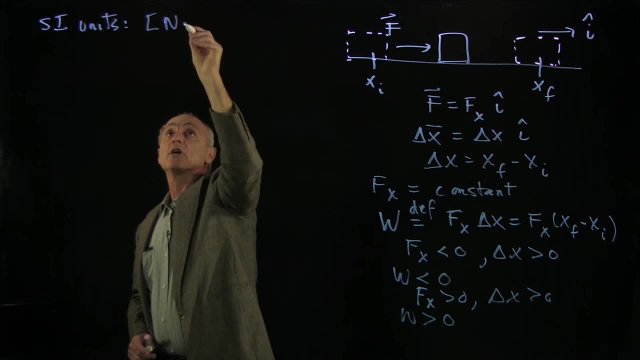 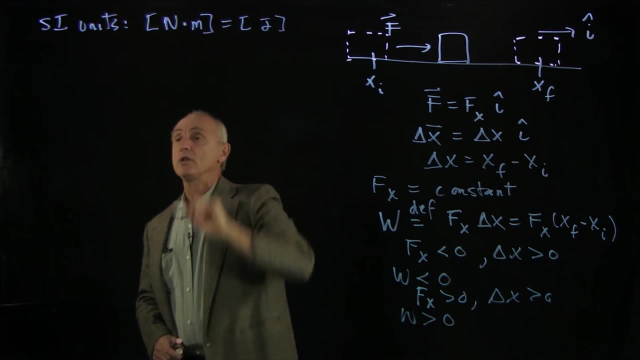 are the units of force, which are newtons times the units of distance meters, And we call this a joule. So 1 joule is equal to 1 newton meter. Now, graphically, we can make an interpretation of this. 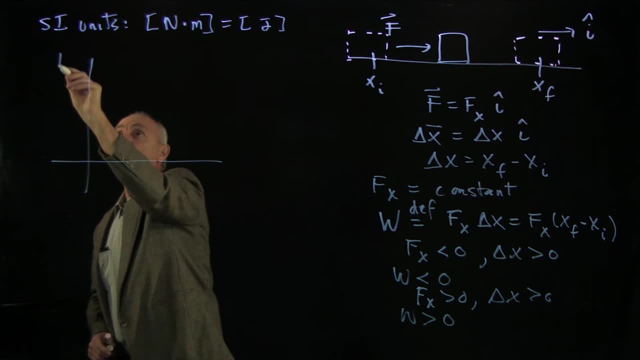 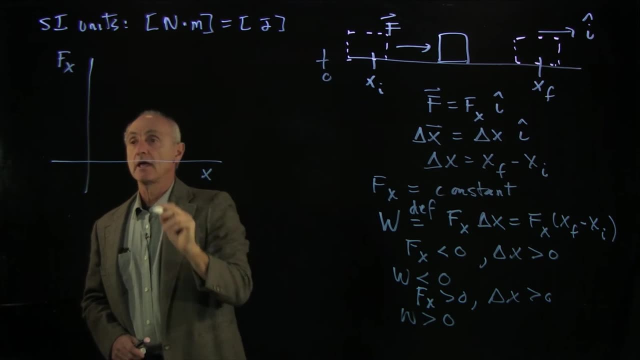 Let's draw a graph of force, the x component of the force, And here, if we had some origin, we'll have x, And our object is starting at xi and it's going to x, final, And throughout this process we're.